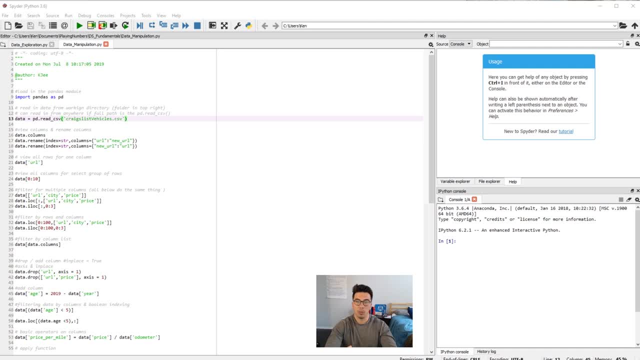 something that is clean enough to get a good output out of. In the first two videos I talked about data exploration and data manipulation. You can see links to those in the description below. You don't need any of the information there to follow along with this video, but it wouldn't. 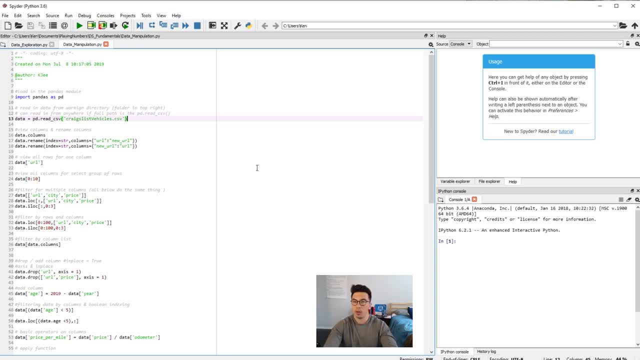 hurt to go back through those, just so you're familiar with how I teach and some of the things that I teach. So let's get started Now. as usual, if you enjoy this content, please hit that like button, And if you'd like to see, 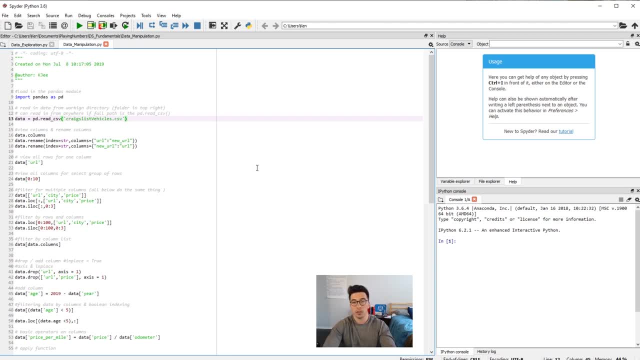 similar videos to this. please subscribe and turn on notifications so you can know when I publish new material. All right, so we'll be using the same dataset as my previous two videos. This is a car pricing dataset from craigslistcom. There's a link to that. 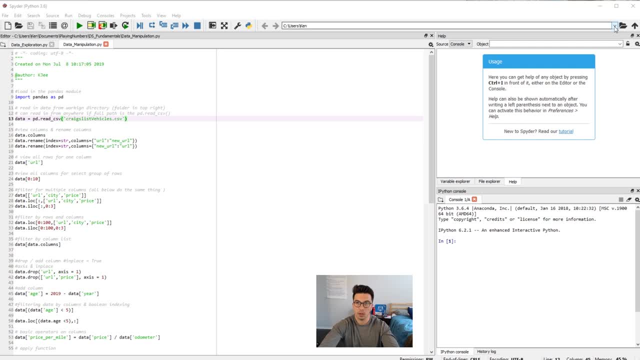 in the description below. I got this dataset off of Kaggle so you can go on there and make an account and download it. I'm going to set my working directory to the folder that has this information And the first thing that I'm going to do- 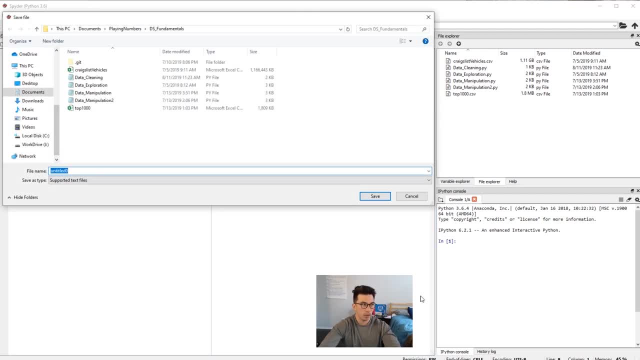 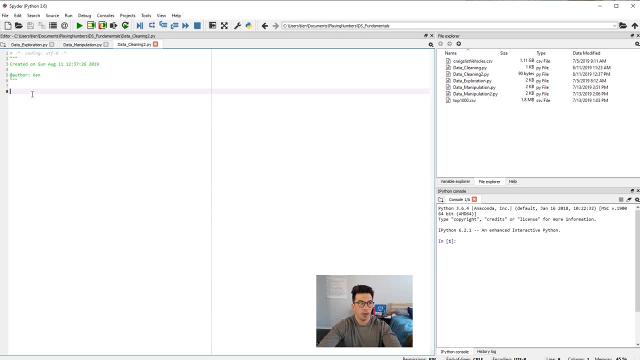 is also create a new file. So I'm going to save this into the same location. We're going to call it datacleaning2.. And now we're ready to get going. So, as usual, the first thing that I'm going to do is I'm going to import pandas and alias it as pd. 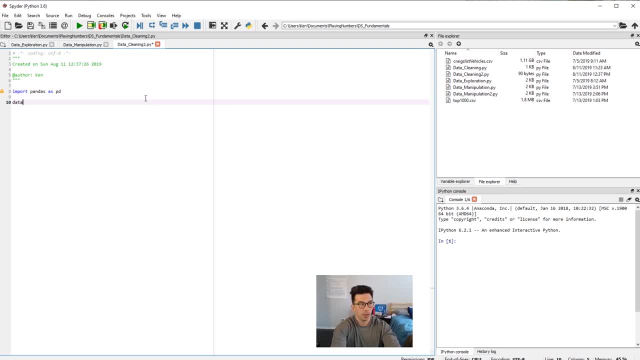 So that we can go forward using that. Next, I'm going to read in the data, So we do pd, read csv, And I like to just copy this name. saves us a little bit of time. Great. So when you see me highlight it, I press control enter on Windows and that actually runs. the 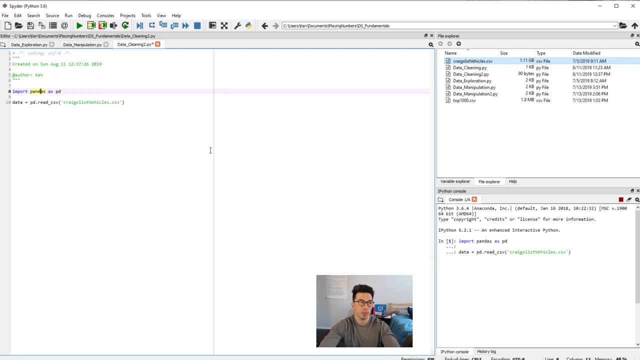 that's a question I've gotten asked a reasonable amount in some of my past videos, so I believe it's command enter on Mac to do that. that lets you just run one portion of your code rather than pressing this button and running the whole file. so now that we've read this in, we can see the data frame in our in. 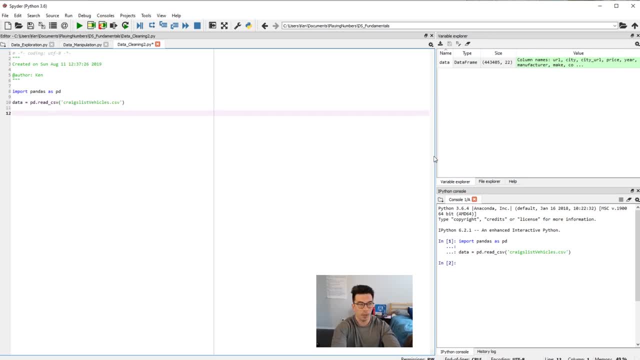 our variable viewer here. so a good practice for me is just to look at the columns- so we've done this before. we can see what all of the features are in our data set, and then we can also do data describe, where we can see all of the 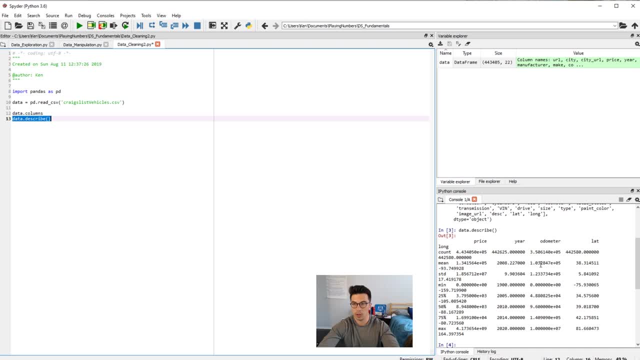 characteristics of the numeric fields in our data set. now, this data set: I've already looked. it does not have any duplicates. but if I wanted to remove any duplicate data I would do this. so we're gonna remove duplicates and then we do data describe, dot drop duplicates and we're gonna do: in place equals true. so that means it's. 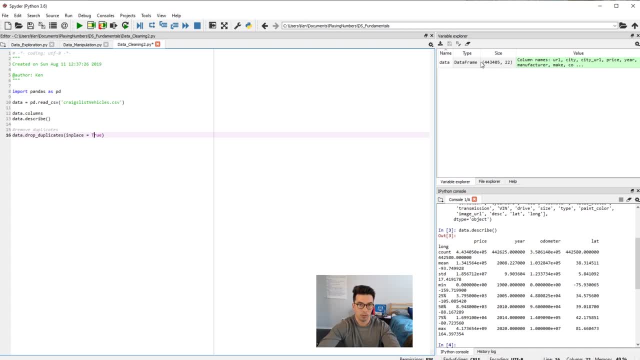 going to use our data set here and drop all the duplicate rows from this one. so if I didn't have the in place equals, true, this would initiate a new data set and I could set it equal to, like data set two, but it wouldn't affect the. 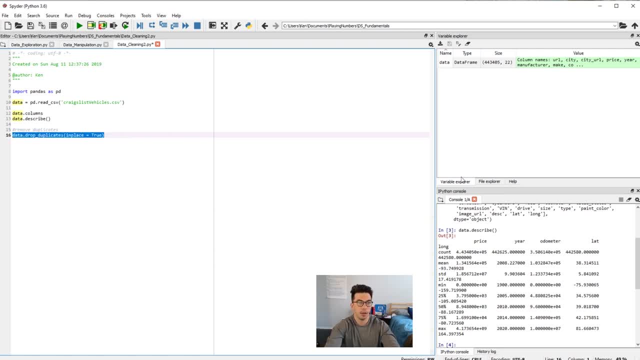 existing data frame that we have. when we do in place, it affects the existing data frame that we have, so I don't expect again there to be any duplicates there. now the next thing we do is we check for null values. a little bit of this is review from our data exploration, but this really builds on itself here and 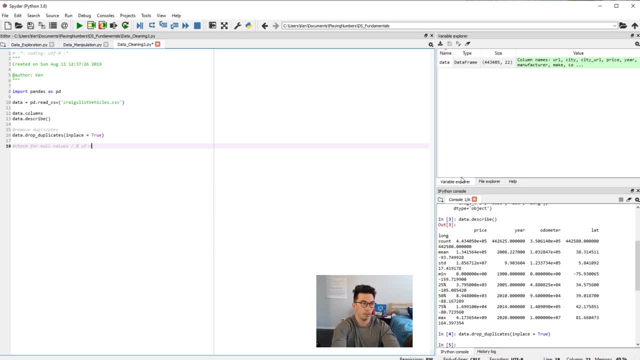 we're also gonna look at the percent of null values that we have. so we can do: data dot is null, and so if we just want to do this, we're gonna build each of the values we're going to need in an, And so if we just were to run this, we would get in each column, each row, if the value 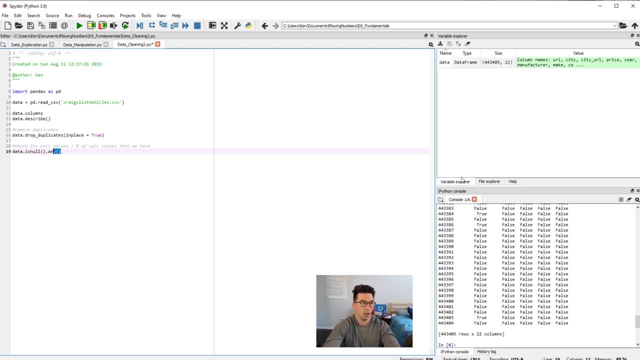 is null or not, And so here we can include the any method and then we can see for each column if there are any null values at all, And so you can see URL. I believe URL is the primary key of this data set. 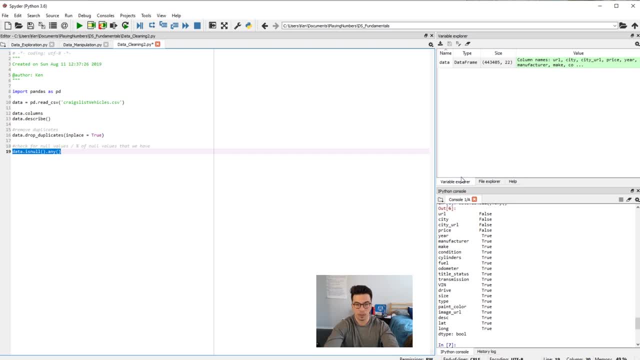 So there shouldn't be any nulls of that. And then we have city, city URL and price. So it looks like for a Craigslist car ad you always have to include a price. That's a feature that they have. All of the other ones appear to be optional. 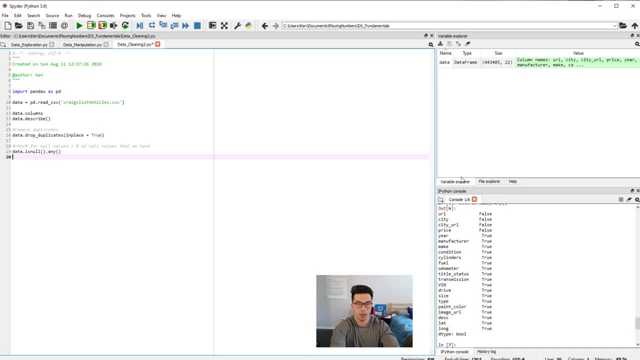 So we can also look at the percent of each of these columns. that is null, So we do data, same thing is null. And since these are trues and falses, when we just do the is null portion. true is equal to one in Python and false is equal to zero. 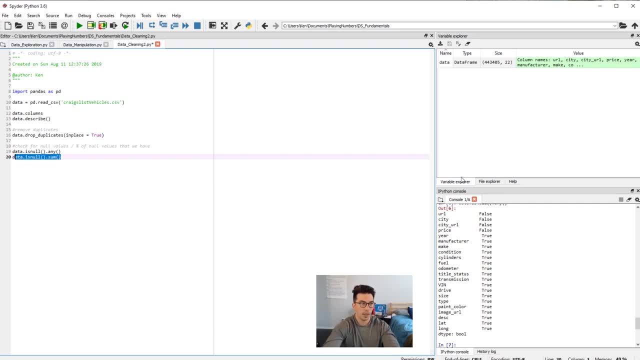 So we can do that, So we can do sum and we can get for each column how many of the characteristics are not null, right? So basically, all of the characteristics in the URL are not null. Actually, it sums up how many are null. 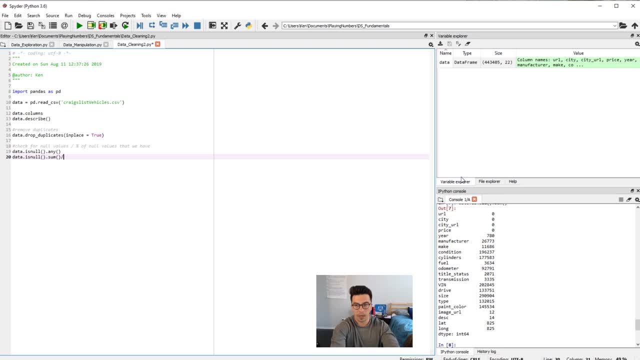 I apologize. So if we divide this by the total number in each column, so we can do datashape. So if we look at just datashape, it gives us how many rows And how many columns, right, So we would want to take the first one, which is the number of rows. 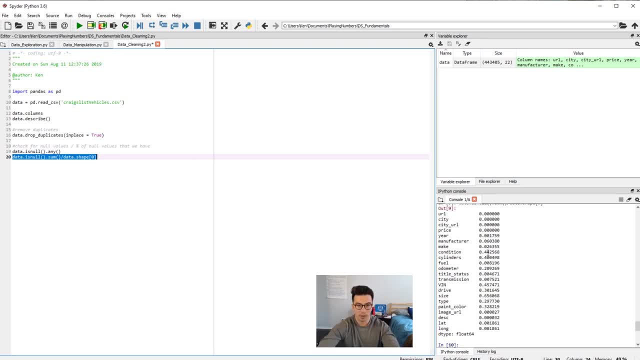 And that gives us the percent of each one that is null. So very few null ones in year, but there's a lot of nulls in the size of the car. Maybe that's a bit more of an ambiguous field. Now, the first thing I'm going to show you, related to nulls, is how to remove columns. 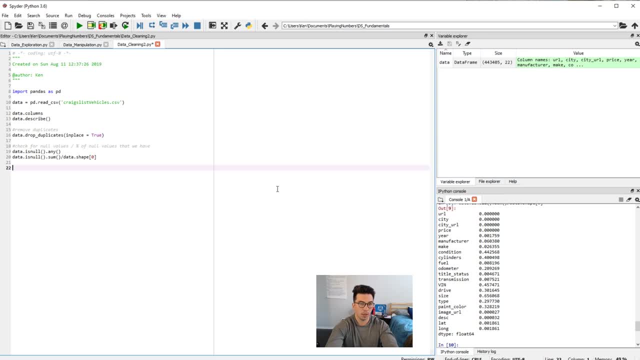 or rows that have over a certain threshold that you wouldn't want. So let's say, a column has, like size, over 65% null. We might not want to include that in our data set unless we were saying, hey, you. 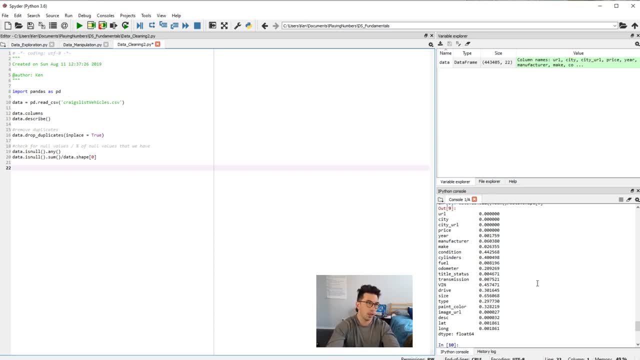 know this is a meaningful feature- if they include size or not, or you change it into a binary or a small categorical variable. A lot of the times, if there's a really high percentage null- you're looking at like 90,, 95%- you might just not want to include it at all. 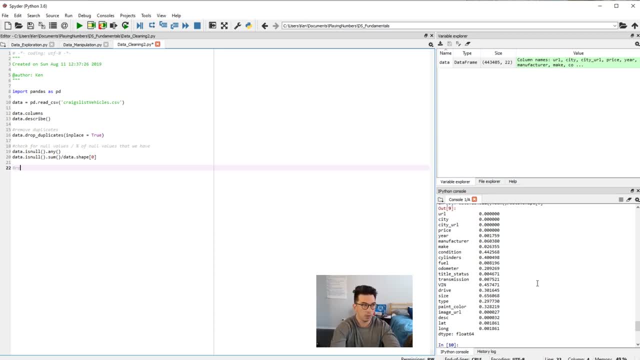 And this is how we would handle that. So we're going to, in this one, remove null columns over a threshold. So we're going to make a threshold and we're going to say we want less than 60% to be null. 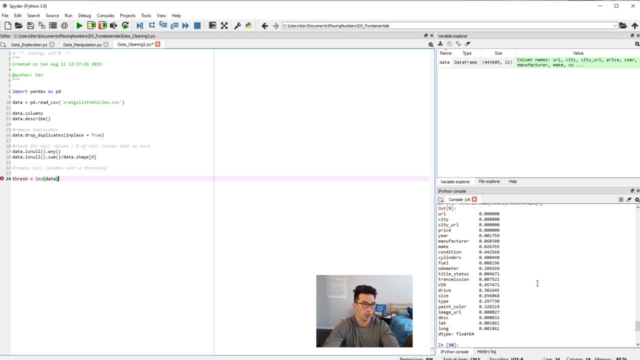 So we can take the length of the data frame, which is going to be the same thing as that shape number. It's just a different way to do it. I like to mix it up just so you guys have a bit more variety in how you can issue commands. 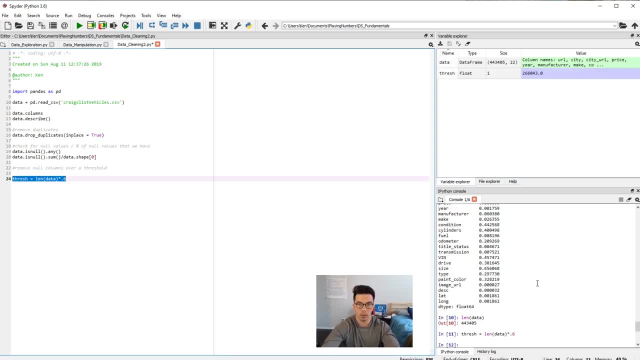 And we're going to multiply that by 0.6.. So this threshold looks like that's around 260,000 of these rows should be not null, And so we can now do datadrawna and we're going to set the thresh equal to our thresh variable that we had above. 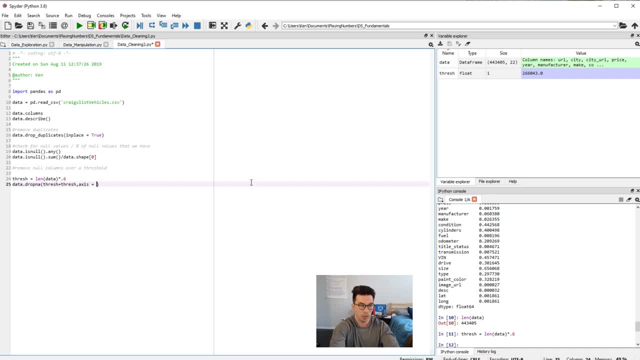 And it's important here that we set the axis equal to 1.. So in my previous videos you know that the axis is if we're looking at the columns or we're looking at the rows. So in this one we want to drop the columns that have a threshold lower than this. 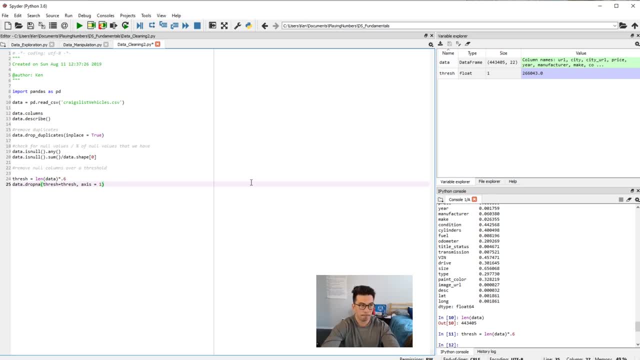 And so, again here, we did not use the in place, So you'll see, the data above is not affected at all And we have this data frame that we output. So we can do on this. let's do shape and see if it's different. 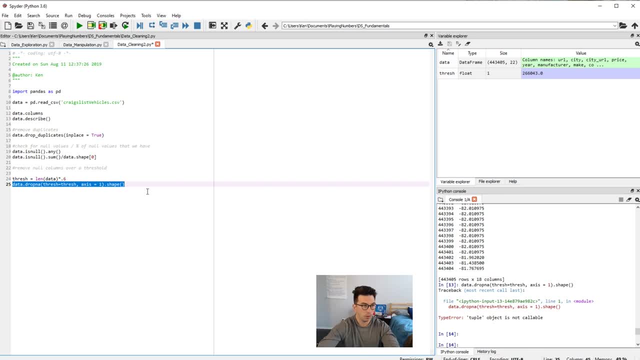 And the one above. Oops, Ah, sorry. So, as you can see, we dropped four columns because four columns were above that null threshold. We can also drop rows with, you know, less than a certain threshold as well, So we can do datadrawna thresh. 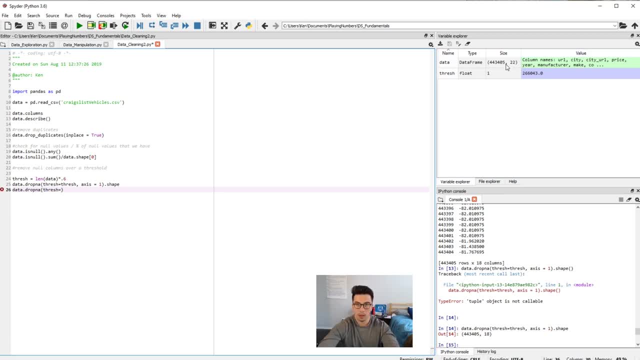 And then, since we have 22 columns up here, let's say we want a Data frame where all the rows have at least 21,. uh, 21 values that are not null, So we can set the threshold. 21 axis is equal to zero. 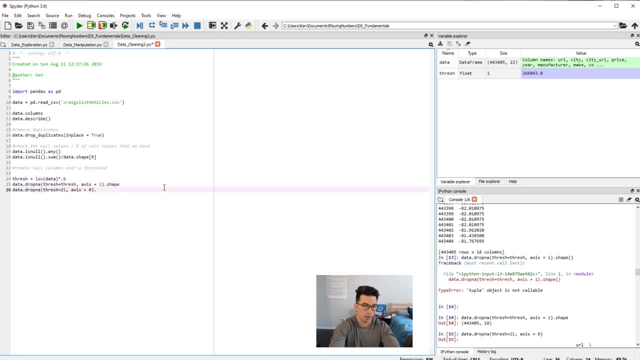 So let's give this a go As you can see it all out. but let's do the same thing with shape, and we'd expect to see significantly less in the rows. value, Exactly. So this cut our data set by almost three quarters. doing that. 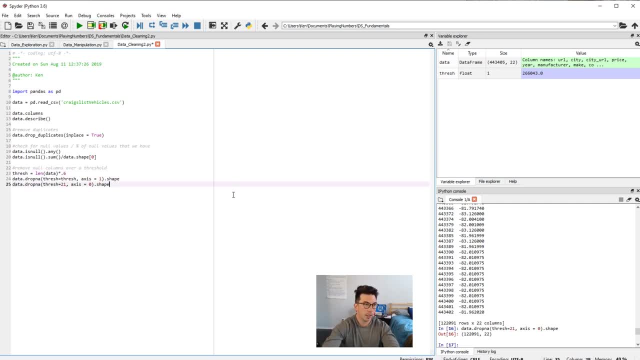 We have a couple options. We can either Drop nulls or we can impute them so we can fill the NAs with a different value. So sometimes it would make sense to fill it with zero. So let's say that in a categorical variable we have a lot of nulls. 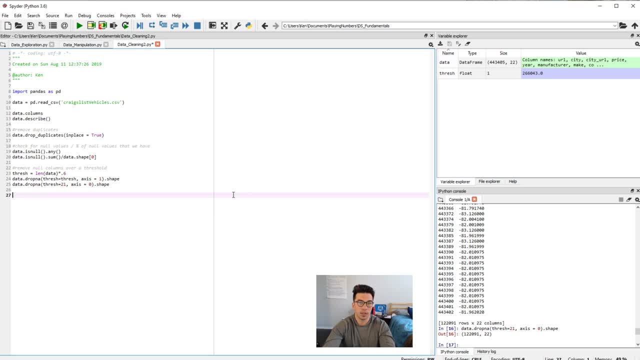 We can actually make it that we can use that as a feature to say, if they didn't respond to this question, that could be meaningful. We can also replace that with the average of all the things in the column or the medium of all the things. 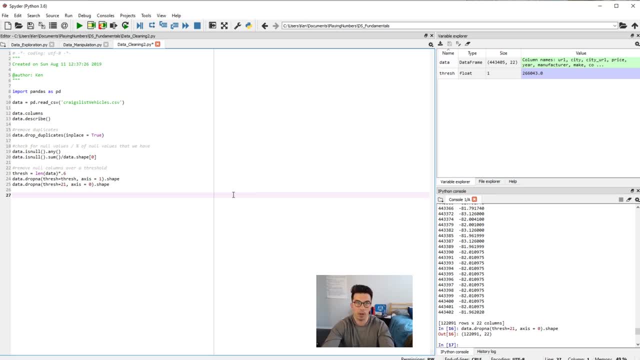 In the column- And this is part of the feature engineering. that can be fun. that can help you, uh, improve your model. So the decisions you make here can have an impact on your model. I usually go through a couple of different versions of this. 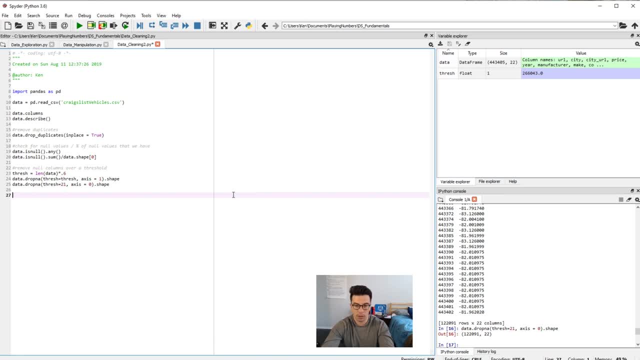 So I'll look at the mean, the median. uh, we'll look at quartiles, different type of quantiles, et cetera. So I'm just going to show you here how to replace a numeric variable with the median or average, if there's a null in that column. 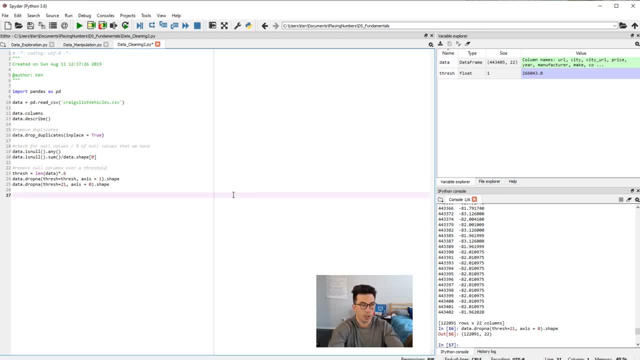 All right. So What we're going to do here is we're going to look at: um, let's see here, Let's rerun this percent null here. So I know odometer is a numeric variable and we can see that from when we ran. describe. 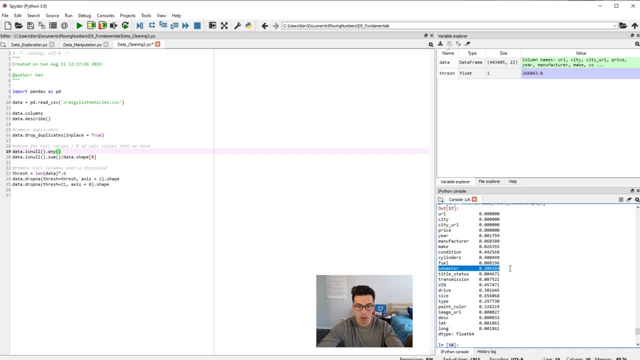 So if we're looking at that, we can say, okay, I want to replace all of the null values in odometer with with something, something numeric, So we can run it through our model. So the way I would go this: 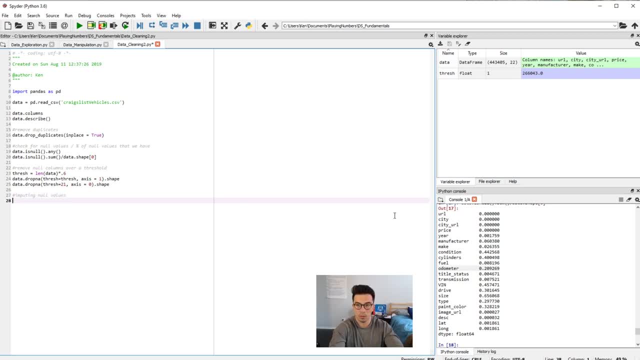 I mean no values, is we just do data odometer, Spell that right? Find out real quick. I did great Uh. and then we just do film that, fill in a, so it just will fill all of the null values in that column with data dot odometer dot media. 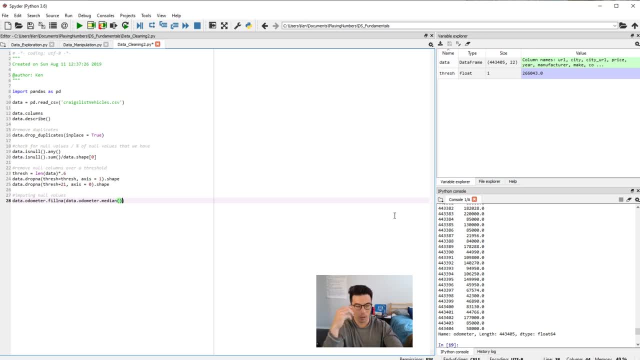 So I like median. It's a bit more normalized if we have like really crazy values Which we might- and we'll find out a little bit later how to evaluate and look for that. So here now we have: if we did this in place is equal to true. it would fill it in the actual data set. 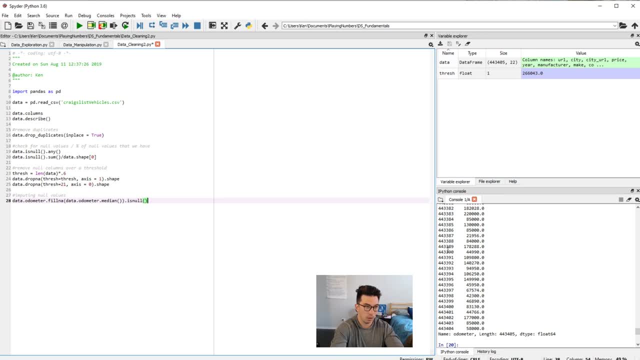 Um, we can do now is null and then any, and we shouldn't have any null values, exactly. So it's perfect with false on the null values there. So we can do the same thing. We can put a function in here As median. this median is just the built in pandas function. 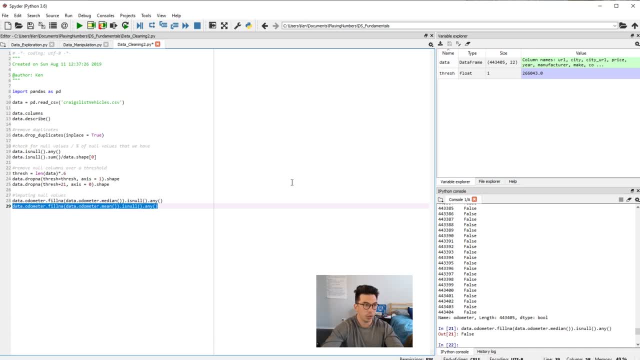 We can also do mean and we'll get the average imputed in there instead. So that's a great way to replace that data. It's a very common approach to handling null values. So, moving on from null values, I think it's always interesting to manage working with some text in your data set. 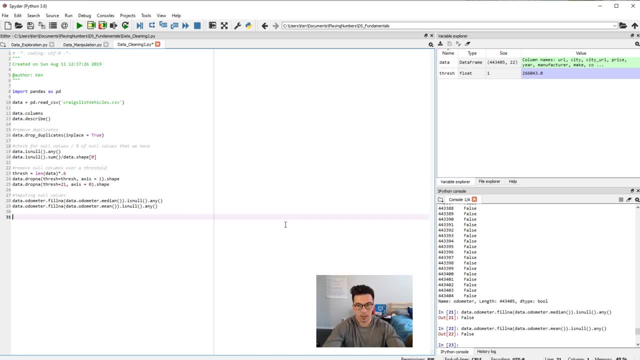 So in this specific data set We have like a description field, and the description field has a mix of capital letters, lowercase, numeric et cetera, And if we want to be able to evaluate that as effectively as possible, we should probably make all of the letters lowercase or uppercase. 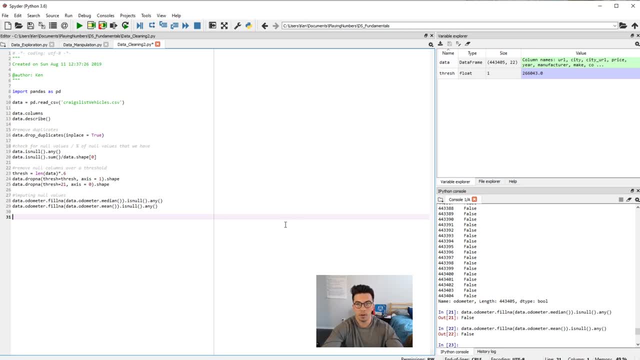 That means if we want to use a bag of word, if we want to use some of these other techniques, everything is normalized. You can't really get rid of spelling problems, but this is a great way to make your data as similar as possible. 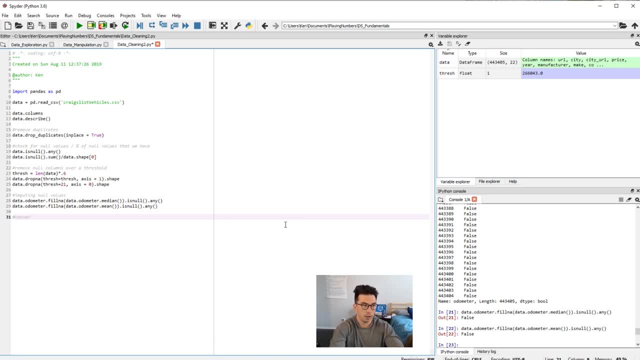 So we're going to Convert here to all lower or upper. So let's just take a look at data Description. So it's D S, C And we're going to look at the head of that Right, And so that's just going to give us the first five. 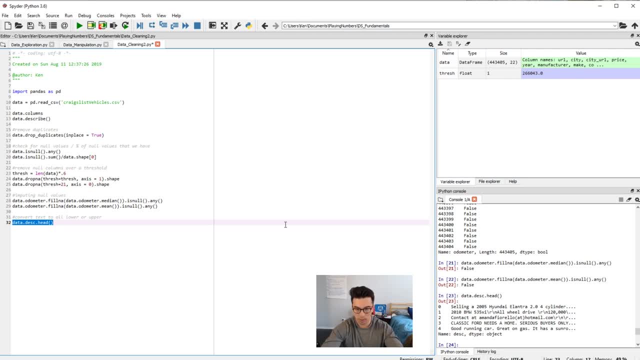 So you can see selling BMW, all of the other. A good example is we have classic board needs a home. That's all capital. that might look different in some of these different algorithms, So we want to Just turn all of this into a lowercase set. 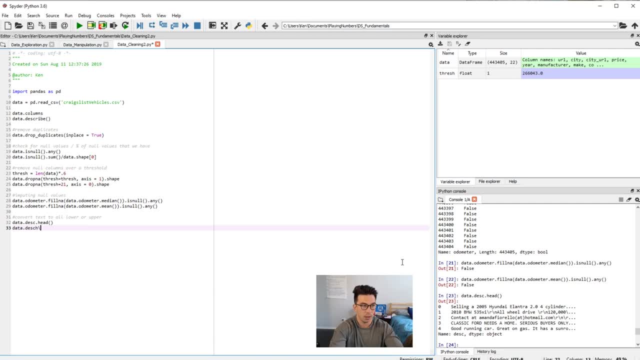 So what we can do is we can be data Descending Dot Sorry. we're going to apply a lambda function, which I've talked about in some of my previous videos. This just basically lets us write a really quick function and apply it to the variables. 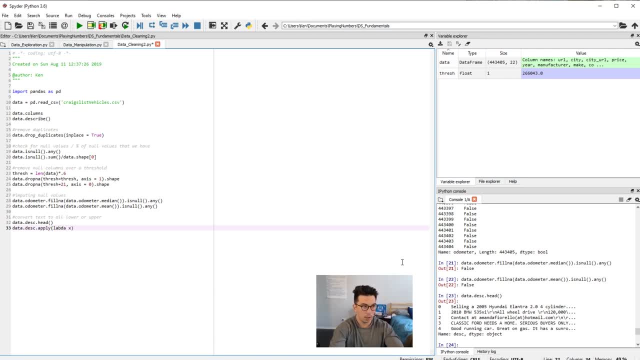 So do lambda, Lambda, Lambda, Lambda, Lambda, Lambda, Lambda X. Now we do X dot lower. So that just converts all of the text in X, which is our row to lowercase. So let's just do the head of this here. 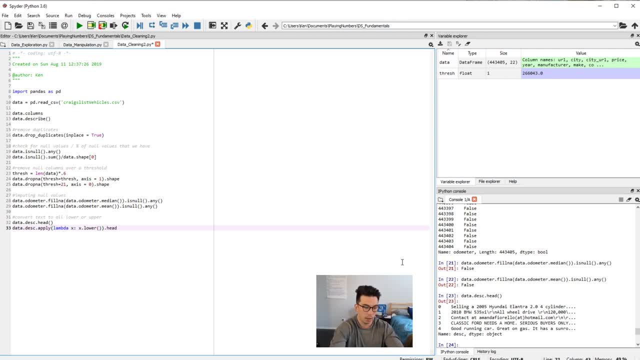 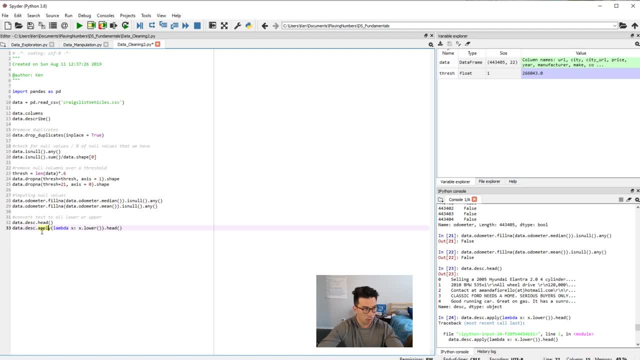 No, No, No, No, No, No. It looks like there are some numeric values in here. That's another data pre-processing thing that we'll have to do. I know that there aren't any lower cases in the head of that data frame, so let's just. 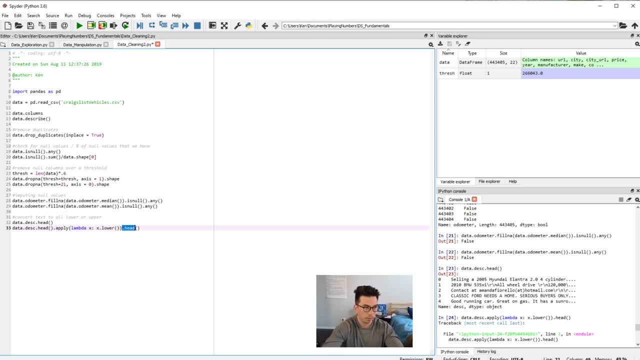 look at the head and apply the same function. Good, So we can see this eliminated. all of the uppercases is that we were seeing before. we can do the same thing. the other action, where it's going to be lowercase, where we change this to upper, there we go and it'll change everything again to uppercase. 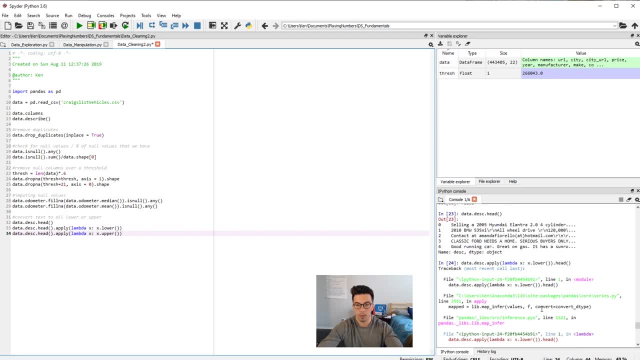 now you saw that we had kind of a type error before. that's something that now we can go into and talk about. okay, how do you manage the, the type errors? so we had some float. it looks like that means that a new, there was a numeric value. uh, adjust a numeric value here, going from float. 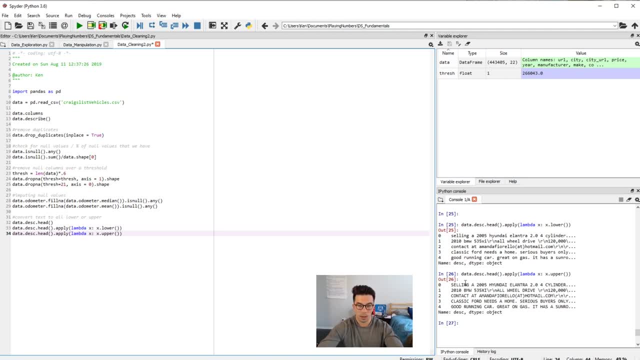 to string is pretty easy going from. uh. i mean yeah, going from string to float can provide some more complications, so let's just handle a quick from like floater into string. so to string. so we can just do data description dot as type string and then we can just do data description dot as type string. 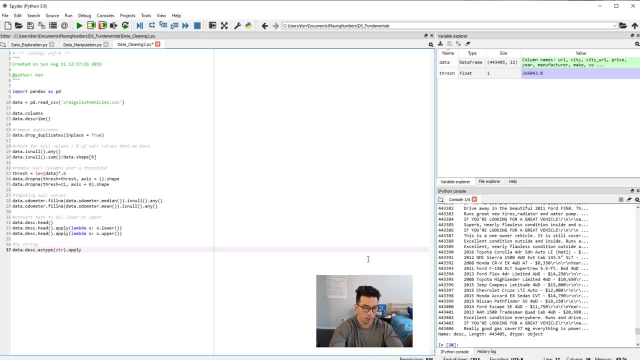 and it'll return everything as a string. so we shouldn't have the same problem that we did before lower, and that should work again. unlike before, where we had some of those issues, it now works because it is classified this all as a string. we can see this by doing datad type and it'll show. 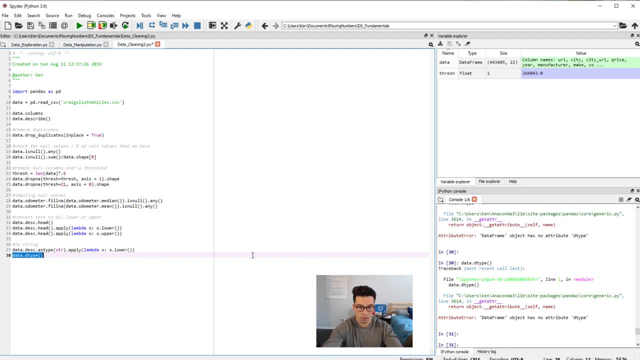 oops, there we go. so datad types, and it'll show the type of all of these things. if it is object, it can be a mix of string and float and int or some of the different types. so we want to make sure that in a circumstance like this, we set a hard rule about what it is and what it should be. 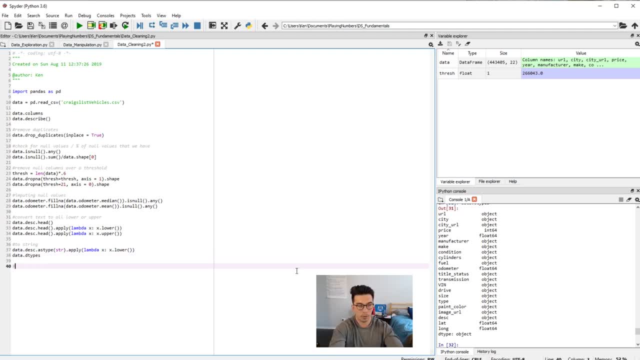 going the other way. this is a pretty, like almost textbook picture, perfect example of how you might want to go from string to uh, in or float. so we'll do to float. so we're going to look at datacylindershead so it looks like we have four cylinders, six cylinders, eight cylinders. you 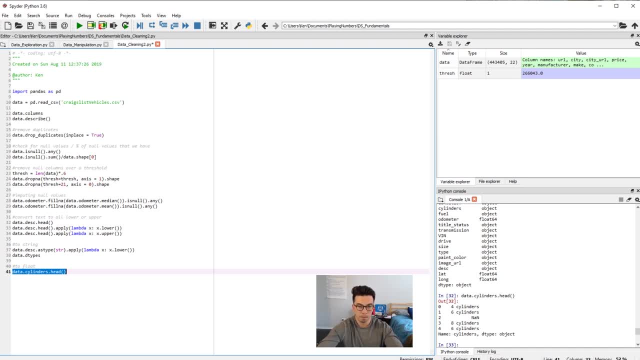 know six cylinders, again, etc. and we also have some non's in there. if we want to to understand this differently. a lot of people would say like why don't we just sort of go with a string and float, just use four, six, eight, why don't we actually keep them numeric and we're gonna go through some? 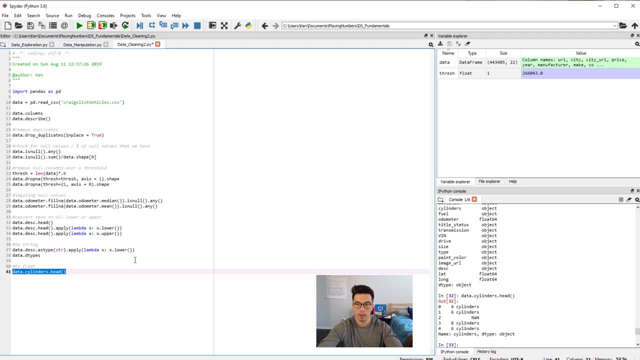 code about how to actually clean this up and make it just a numeric uh type. so i'm going to do that now. we're going to go to datacylindersd type, just for a little background. so we know that it is an object, so that means it can have like a mixed type. we're also going to do data cylinders. 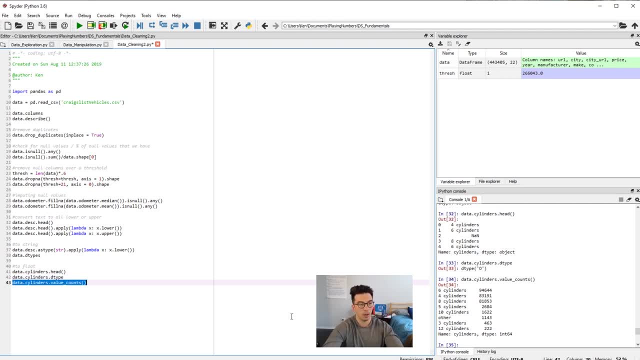 value counts, just to see how many are of each different type. so we have other, we have, you know, three, four, six, eight, five, ten and twelve cylinders. um, so no 16 cylinder cars in this data set here. i guess they're not selling any mac trucks or anything. but the next step here is that we're going to replace 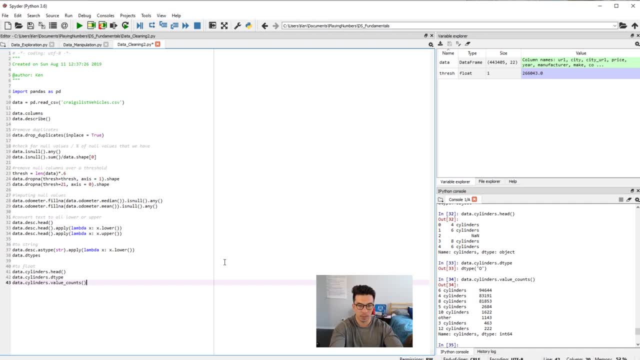 cylinders with basic, basically a blank space. so we're going to remove cylinders from all of these cylinders. uh, that apply. so i like using lambda functions here, so lambda, and then we're going to do lambda x and then we're going to take- um, we're going to make sure x is a string we're going to take, that we're going to replace. 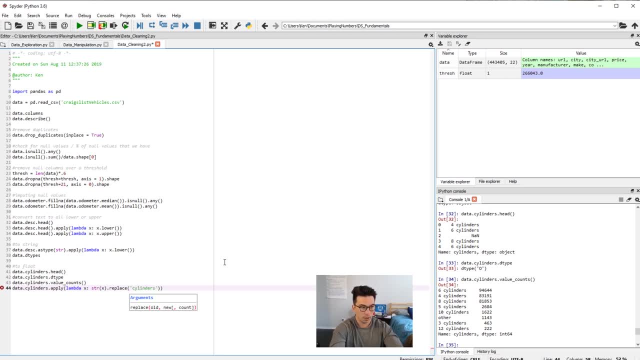 cylinders. so these are all cylinders. we should probably do um, change this to lower right, knowing that it's a string, and then we're going to replace cylinders. just we're doing lower just to make sure that cylinders are all the same and we're going to replace that with just a blank right. 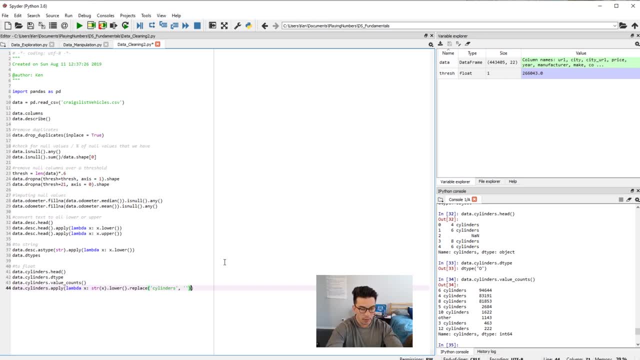 i'm sorry. there we go and then we want to strip this of of any extra. so strip just removes any extra spaces on the outside, so they should clean this out there. just nice and dirty. then we have a string, so we're adjust the beef and for this reason that we want a string, i have an L Extrude box and we want to place this into the composedка. 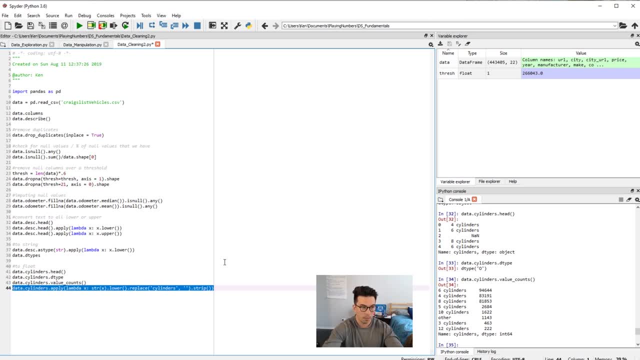 sales institute to machine it. so we've got a U tehd. we do have two less tabs and then we're going to open this up. so we're going to bring this up, we're gonna set up aчеady, then up quite a bit and we want to set this actually equal to this. so this will. 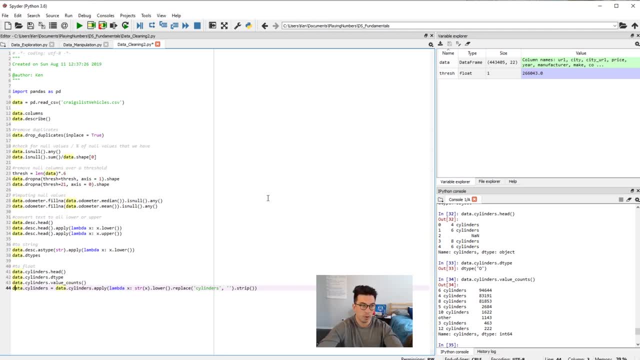 actually change data cylinders in our data frame here so that it has cylinders removed and it has it is stripped of any any extra spaces. so it was actually quick. now let's look at data dot cylinders, value counts and see if it worked for us. nice, so we still have this other that we have to deal with and we 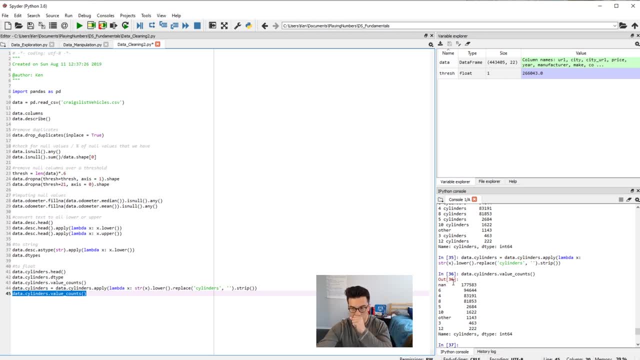 have a lot of null values. so there's a couple different things that we have to do here so we can transform other into nones. I believe by doing this one quick thing here, so we can transform other into nones, I believe by doing this one quick. 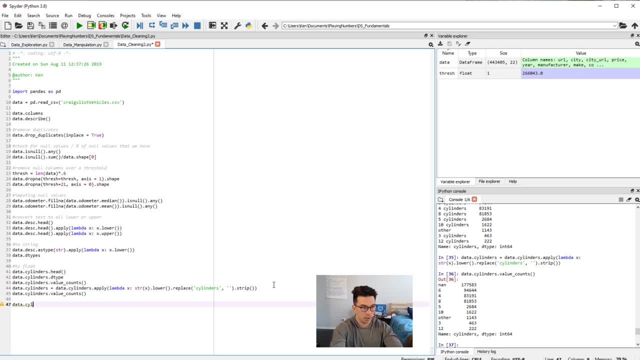 here so we can transform other into nones, I believe by doing this one quick. there's obviously, and there are gonna be errors done, so your rs and they equal. we want to coerce them so that should make them into the correct data type. there's obviously and there are gonna be errors done, so your rs and they equal. 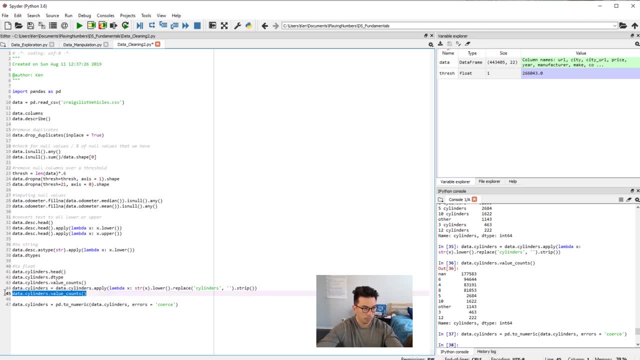 So let's try this one more time. We're gonna do value counts again And now we have a good, clean data set of all cylinders. So the next thing we would do again would be to fill the null values. So let's look: datacylinders is null any. 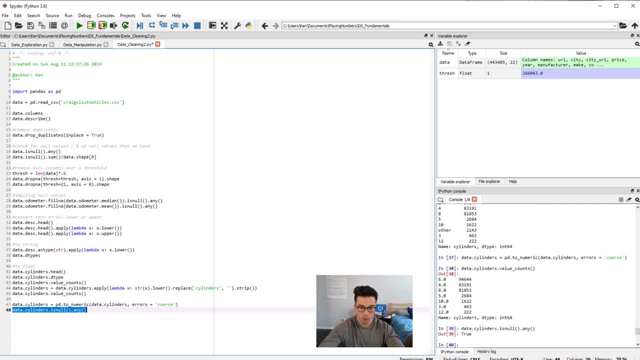 And let's compare that to the null values that we had before. Oops, we wanna sum them, sorry, Cool. so we're looking at 178,000, which seems to be good, because that would include the non's there as well as the other here. 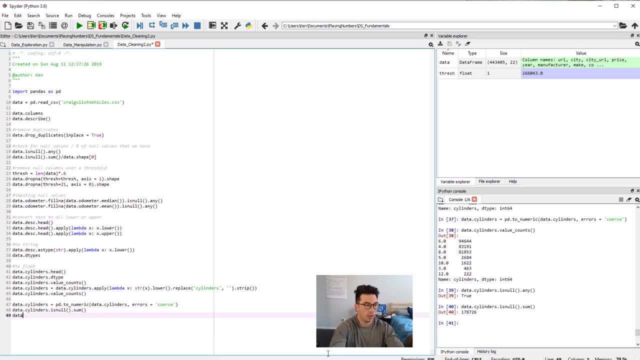 So we can now impute them with datacylindersfill any, And then we wanna do datacylindersfill any, And then we wanna do datacylindersfill any, And then we wanna do datacylindersfill any. 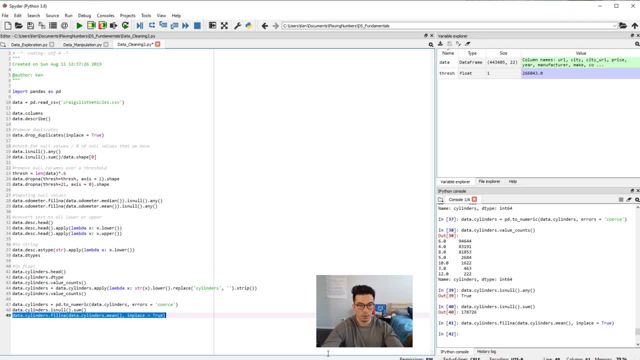 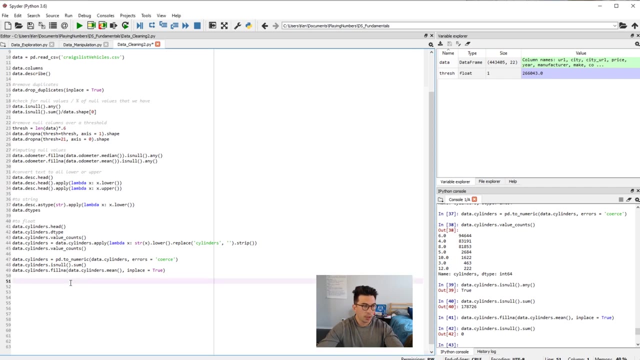 And then we'll do employees equals. true, That will fill all of those data frames there, All of that data frame. So now we should see there's no null values. So when you're actually cleaning data, one of the most valuable things you can use is 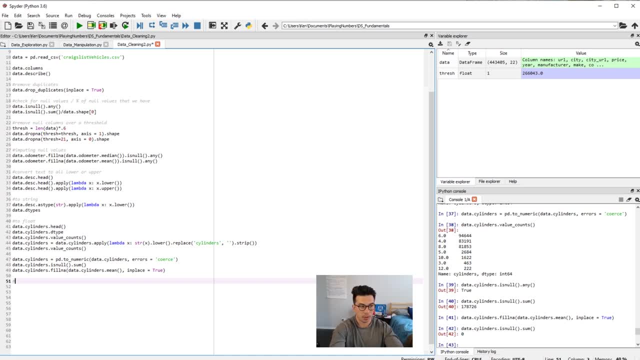 one of the most valuable things you can use is histograms and box plots So they tell you if there's something basically wrong with your data. So let's look at a box plot first, We'll do databoxplot and then we'll look at odometer. 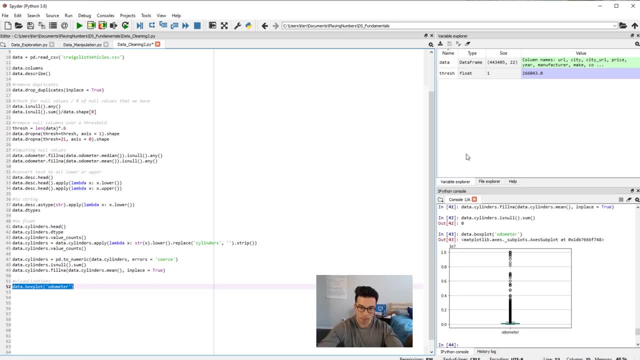 Right, So let's see here. We should see, okay. so there's a ton of outliers that go above here And this is LE. so this is to the seventh. So we're looking at, you know, 100,000-ish more. 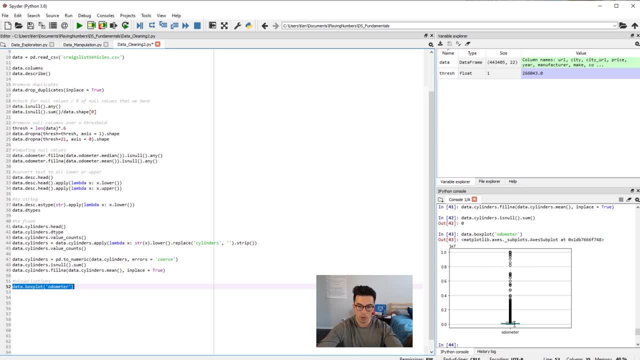 100,000-ish miles. might be more than that, But usually you wanna see a big box, because that's where the main bulk of your data is, And then a couple outliers on the top. If we look at price, I think price is extremely skewed as well. 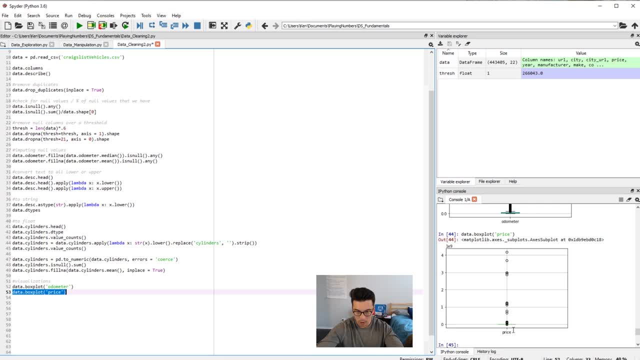 We can see that. you know, the box is very small here And we see a lot of upwards deviation. You know this is like millions, billions of miles, which is probably unrealistic. someone probably fat fingered some things there. so let's focus on 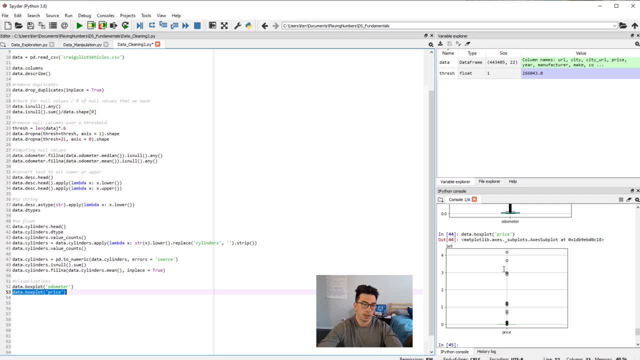 you know, understanding what this tells us about the data. that means that there's some error and we probably want to clean this data set. maybe take, you know, a z score within a certain range, rather than using all of the data points, because this error is likely related to someone mistyping. 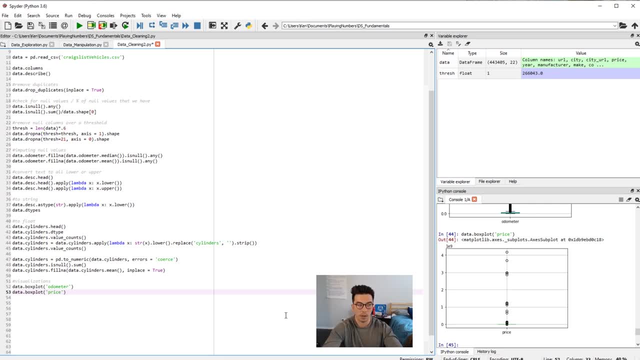 something, not something that is actually within the realm of reset. the other thing that we can use is a histogram, and let's do this for odometer, and so this tells you how many, very how many um data points are within certain ranges. so, again, we have very few that are super high, and that's doing everything to this one bucket here, which 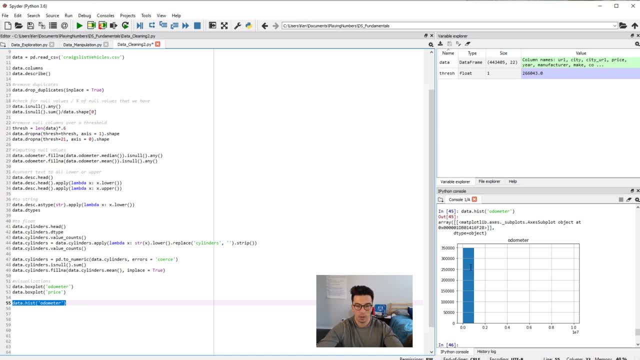 is not what we want. we want a bunch of different. we want to be able to see the actual distribution. so let's clean this data up, let's remove some of the noise by trimming a certain amount of unneeded variables, and then let's do the histogram again and see what that 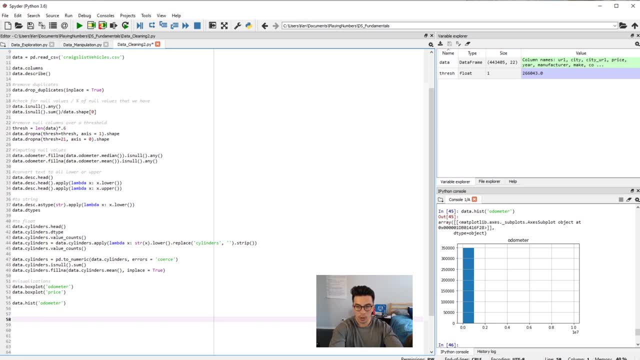 looks like. so we're going to do this only on the numeric variables. so we're going to do: numeric is equal to data dot. this is a kind of a hidden command, so it's get numeric and it'll just return all of the- uh, all of the numeric variables. 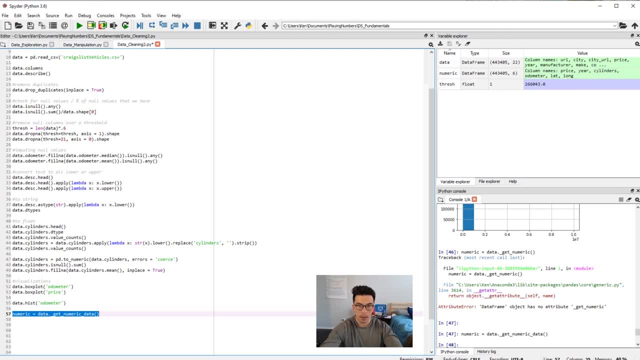 uh, sorry, i need the data, which is a fun kind of little little trick. so you get all six of the numeric variables that we've created- and now that includes cylinders, correct? so this time, if we want to do this for all of them, we're going to import a couple different modules, so we're going to import. 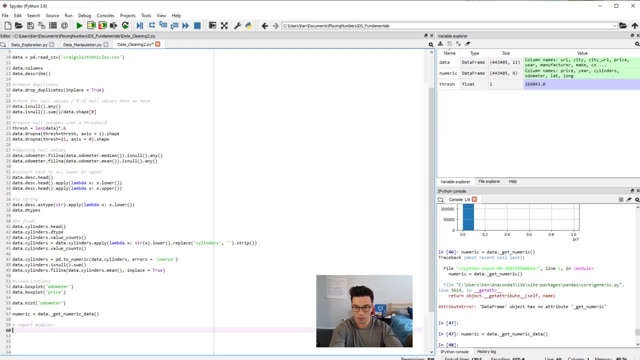 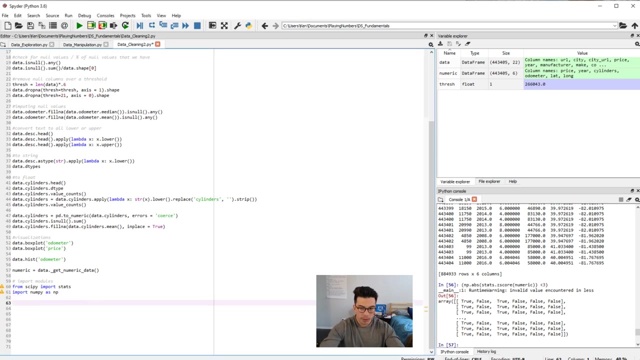 import modules. we're going to do from psi pi import stats and from numpy no, or we're just going to import numpy, import numpy as np, all right. so the best way i found to do this is: let's say we wanted- you'd probably want- to do these individually so you can do data. we'll just make a new data. 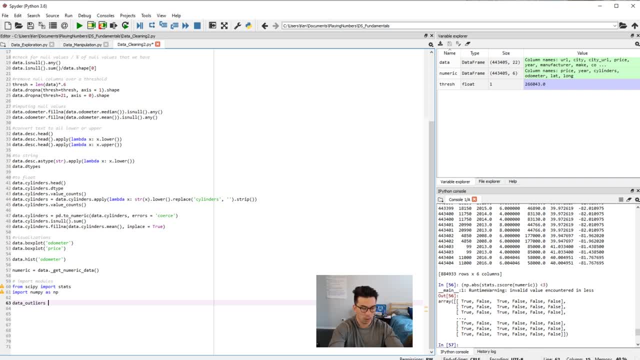 frame outliers and that's going to equal to data. we're going to take uh, data dot price and we want data dot price, dot quantile to be, you know, and then 99.5 percent top right, so it's less than whatever this value is um. so anything over this on the high end is going to be too high for our use case here. 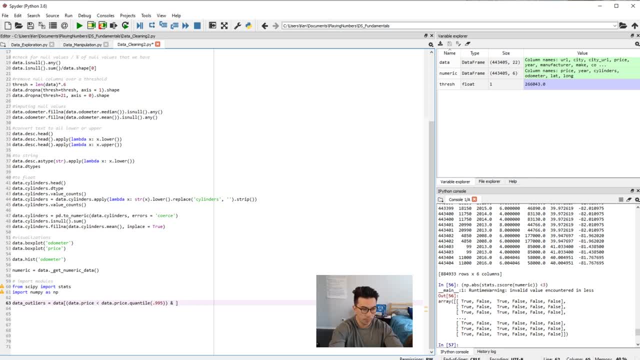 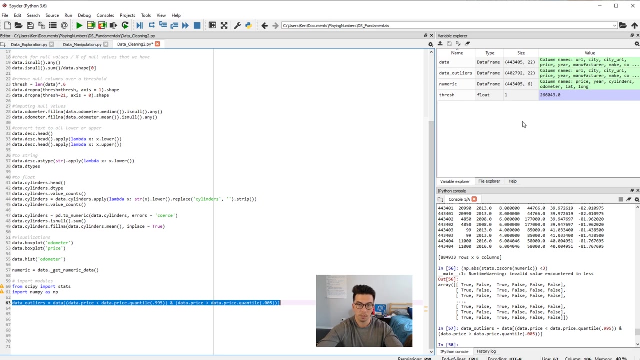 we also want, on the other end, data dot, sorry- price to be greater than data dot dot price, dot quantile, than anything in the 0.005 range, and if we run this we should get a data outlier set. so we shaved off 41-ish thousand rows here, and so that should really reduce the amount of. 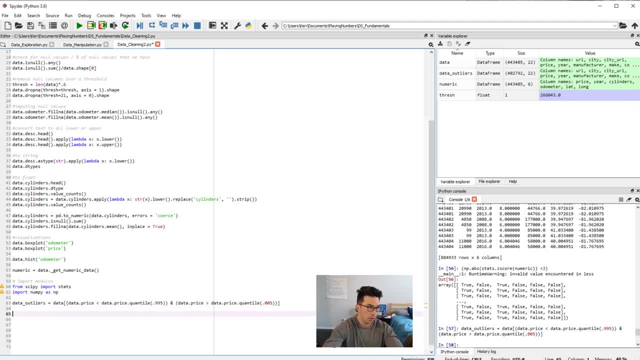 huge outliers that we had. so let's take a look. we just did price, so let's do databox plot and then we'll do price again and see how this looks. so that, oh sorry, it looks the exact same because we did data and not hit outliers. 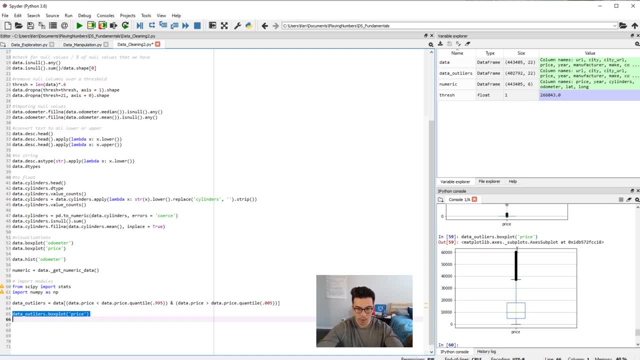 let me worry for a second. there you go. so we still have a lot of upended outliers, but this is the. the mean right here is around ten thousand dollars. we have, uh, i believe the high end is the. you know, this is basically uh, a certain subsection. i believe it's uh like the 25th percentile to the 75th percentile. 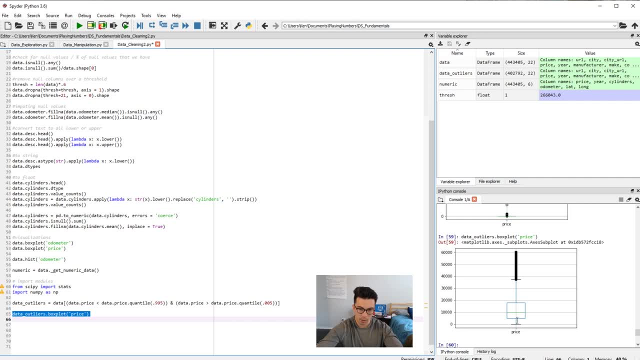 these up ends are the 90, uh 95th percentile, uh like, of the outliers, and then these are anything above that area. so let's also look at the histogram of the of price again as well, just to see what that would look like, because before this is what it looked like before. right, so everything was uh right. 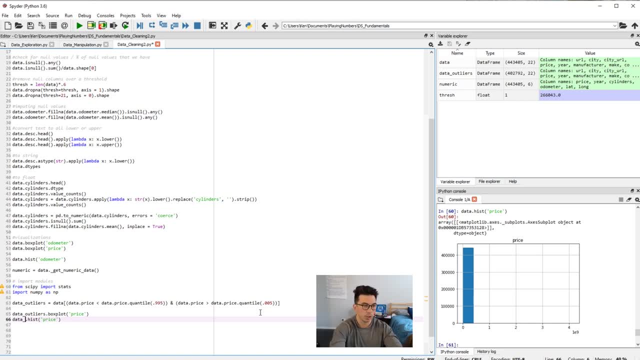 around the left side of the screen because we had such huge outliers. now when we run it, it should look more like a normal distribution or a half of a normal distribution, because we're starting at zero. so that's also something to consider. i'm not going to get too far into it in this video, but 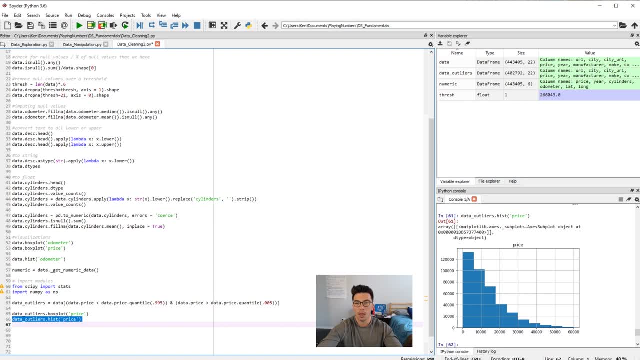 on craigslist it looks like a lot of people just put the price at zero and did like a what's your best offer type of thing. that's something that we might want: to remove all of those in the data set and get something that's more normally distributed, or we want to- uh you know- change how that's done. 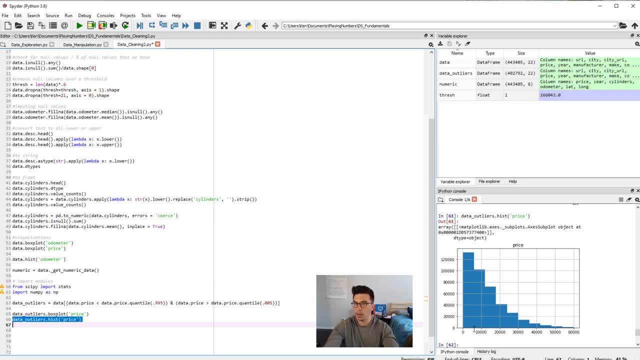 see what if they, in the text, they had some sort of uh pricing information. but it's something to watch out for, something to think about when you're evaluating this data set. let's do the same thing for um, for the outliers with um, not just price with the odometer. 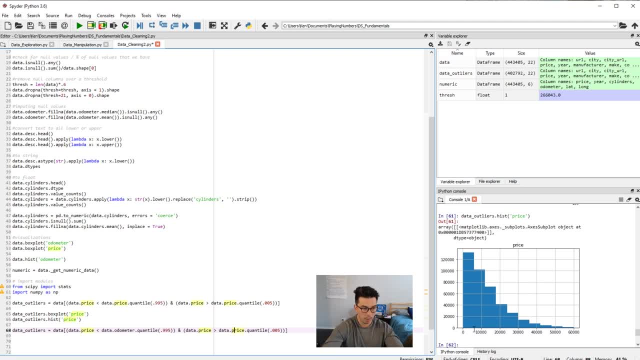 so we're going to change the odometer here, we're going to change the odometer here, and we're only going to change it everywhere, i guess, and if you're going to be repeating this whenever you have to do something more than once, i recommend writing a function. but for this use case, um, for essence of time, i'm not going to. so. 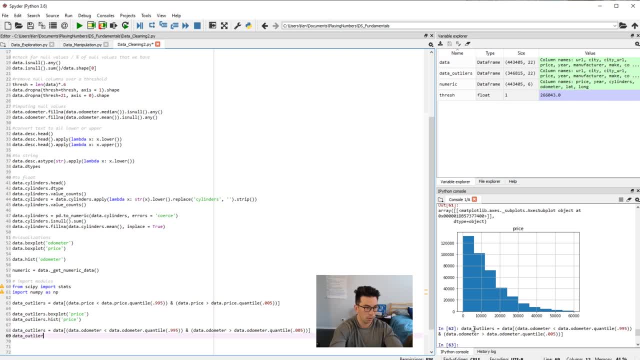 same thing: data outliers, dot test, let's do box plot and then we're going to do odometer. perfect, so we should see something similar again. you have this box plot, which is pretty normal. you know, no one's selling a negative car value, so we wouldn't expect to have too much downside. 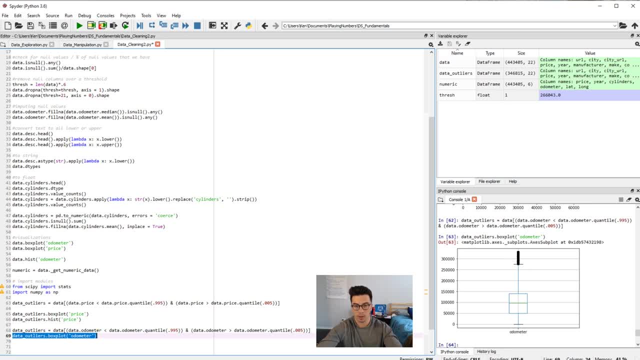 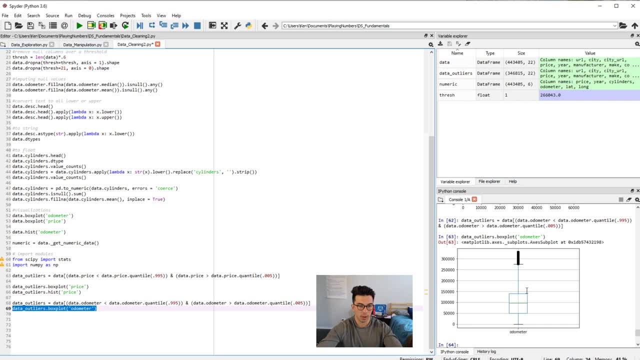 deviation, but there is a good amount of outliers that are above that certain threshold up here. so, again, this is a great way to visualize and understand the data cleaning process and this is how we can go about removing certain thresholds. so we could remove an even larger threshold, we could remove only a top side threshold by doing something just this. but 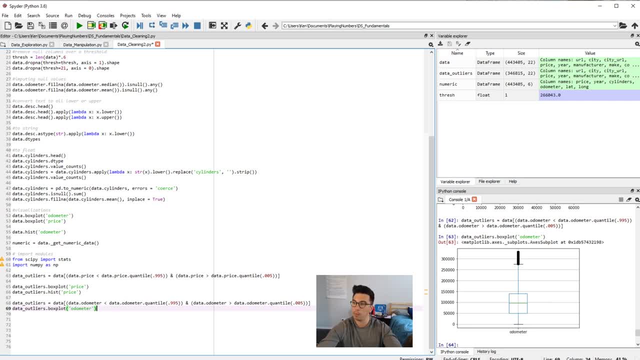 we can't just use this as a default. in our use case, this is a the most effective process right now. so the last thing i want to talk about related to data cleaning is scaling your data. so for some algorithms, especially the ones that use euclidean distance, like k-nearest neighbors, it's important. 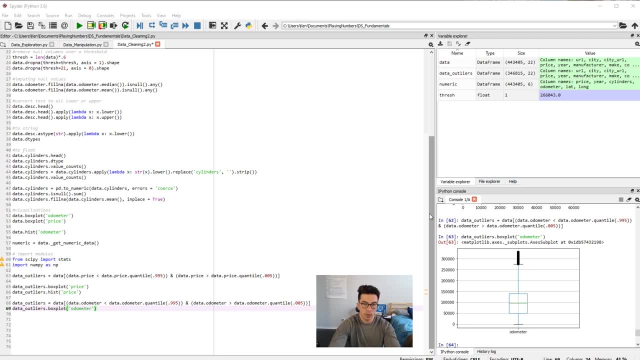 to make all of your data on the same scale. so, again for something that uses distance, larger values can have larger distances when, and that means that some features will be larger than others in the algorithm. so when we scale something, we put everything in the same numeric range. so a lot of the times you'll see like 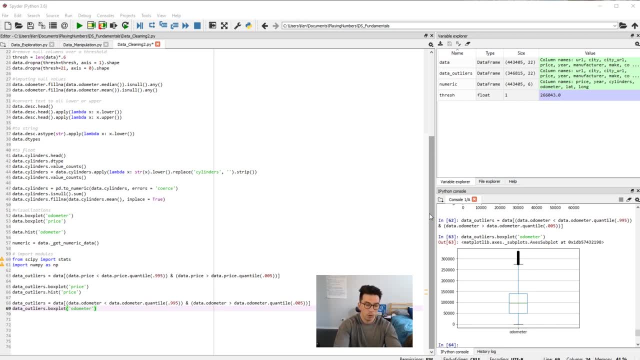 like z-score scaling, where you make everything a z-score, or you'll have, like, i guess, like some sort of mean differencing, which can give you a score between negative one and one, and then you have min max scaler and some other vector scaling techniques that'll give you a value between zero. 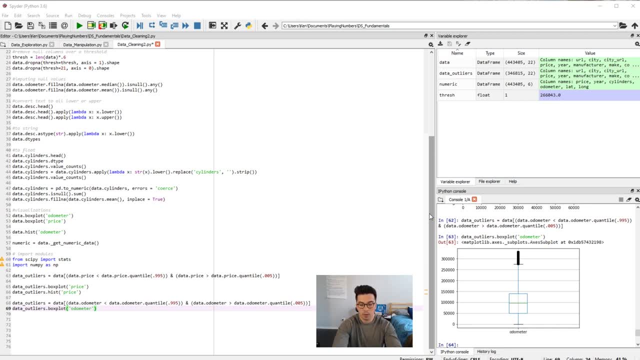 and one. so i generally like values between zero and one. they're they're great for different types of analysis or again, k-nearest neighbors or doing some pca stuff. so let's go through and show you how to do this. you don't generally need to scale your data with linear regression or with tree-based. 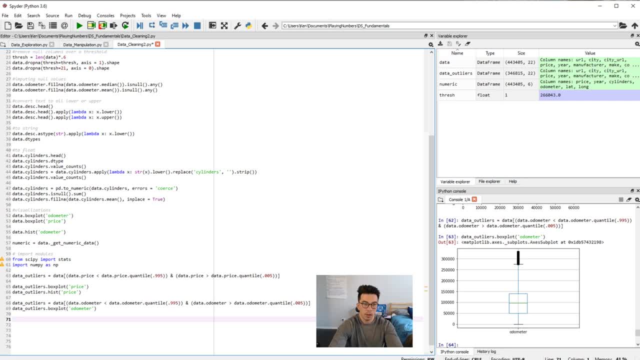 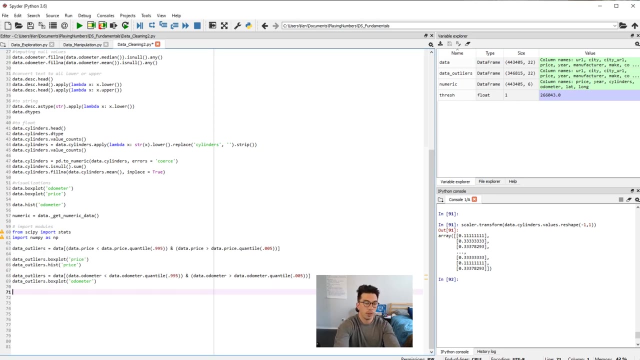 models or, you know, naive bays. but there are some specific types of models, even in deep learning, where speed and quality. so, to get started with min max scaling, we're going to use a different library than we have and we're going to use sklearn, so we have to import that. so from sklearn, 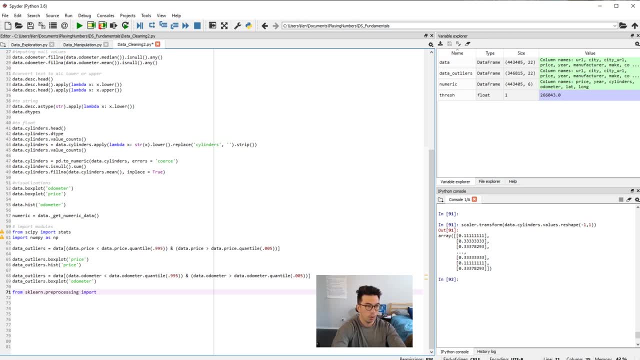 pre-processing: import min max scalar, and we're going to do so. when you do this, you have to create a scalar object and that is scalar, all right. so we fit this scalar object and then we use the scalar object on our data set. so, in order to fit this, we need 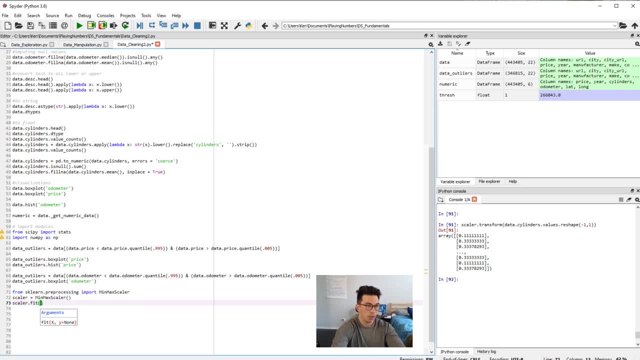 scalar dot fit and we put in the data that we want to fit to it. so it's data cylinders and then. so you have to do some to get one frame fit. you have to do some idiosyncrasies to get it in the format that it's looking for. so we can either use numpy to do this or we can do kind of 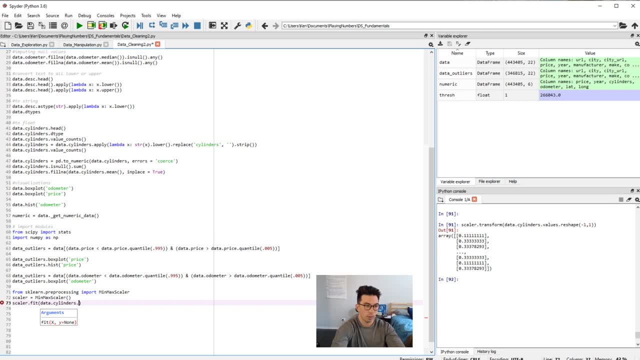 a workaround in pandas. i'm going to do that, since this video is mostly focused on pandas. we do values, which creates an array, so datacylinders is a series. if we do datacylindersvalues, it's and it becomes an array and we have to reshape this array so it's an array of arrays. 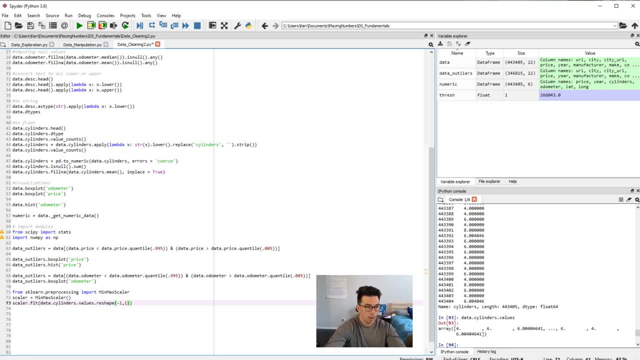 so we do negative one on one, and let's look how this looks now. so it seems like a lot of hoops to go through, but now you can see this is an array of each of these individual arrays that we have. that's just the way that this feature scaling module accepts the data in, so we have now fit this. 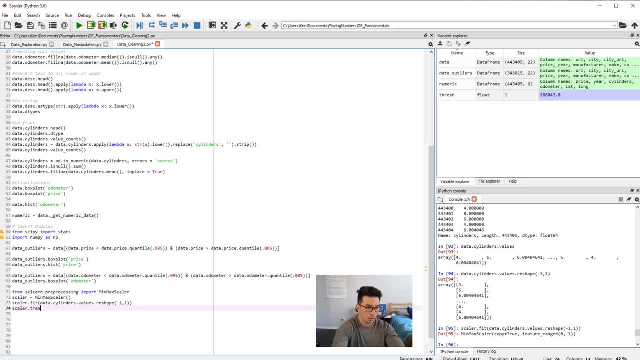 and we do scalar transform and then we do, we copy this same information. so, as you can see, previously we're looking for six, and then this is the average number of cylinders. we should be getting things all now between four, six, and then we should be getting things all now between four, six, and then we should be getting things all now between: 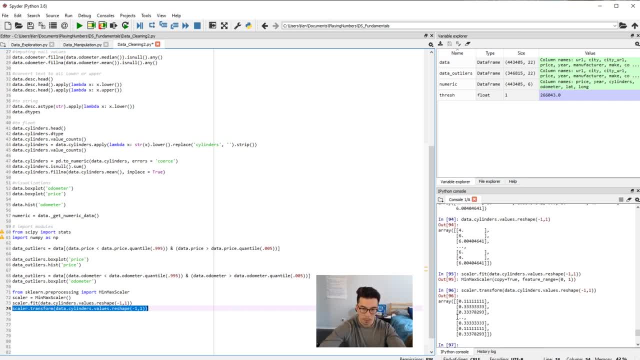 it zero and one, so same thing. now we have ones, and these are all scaled individually. so we can also skip the fit and transform set and we can just do scalar fit, underscore, transform and include the same stuff and we'll get the exact same results, but generally how sklearn? 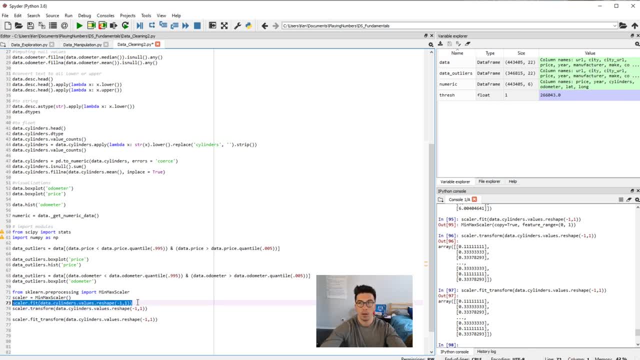 works is you fit a model and then, when you want to find the output from a new input, you use this form feature and that's how they have built out all of their regression, of their machine learning, any of these other algorithms that they use there. so after you've scaled this, you can scale all of 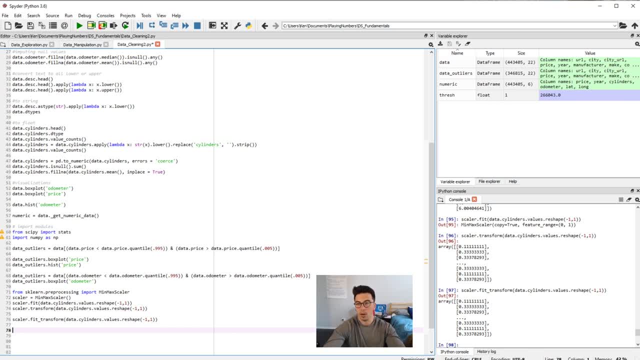 your numeric data, or just some of it again, depending on the type of analysis that you're hoping to run. i think that's it for data cleaning today. again, thank you so much for watching. if you have any questions about this, please leave them in the comments section below. 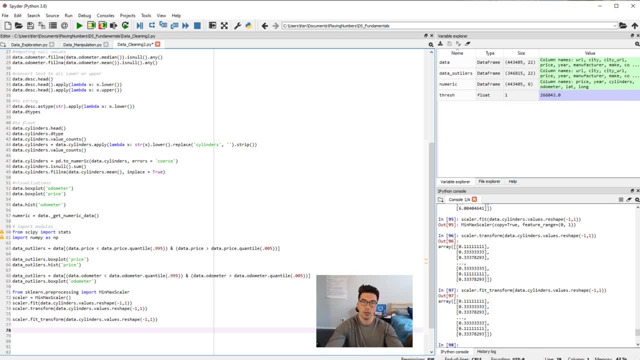 good luck on your data science journey and please look forward to more videos like this from me. 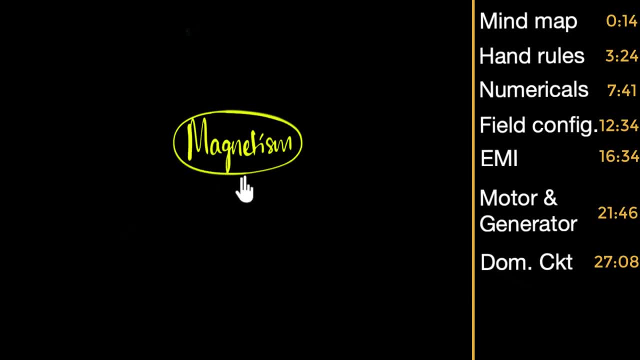 Let's summarize important topics of magnetic effects, of electric current, which, in short, I'm calling magnetism. On the right hand side you can see the index. so if you want to jump to any specific topic, feel free to do that. So let's begin with the mind map. I like to 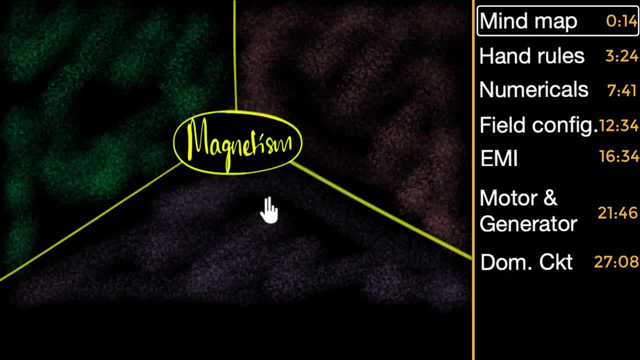 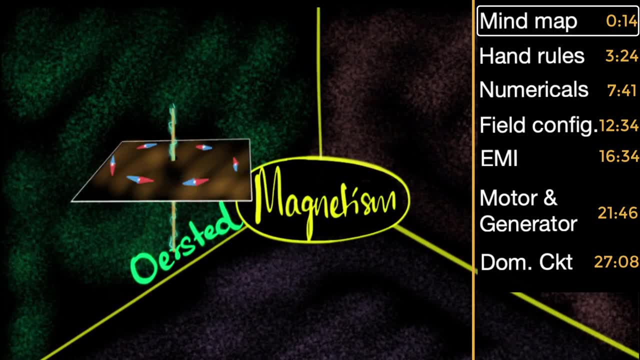 divide this entire chapter into three parts, based on three scientists and three discoveries. The first one is by Ørstad. He discovered that current carrying wires can deflect magnetic needles, In other words, they can produce magnetic fields. This is what laid the foundation.